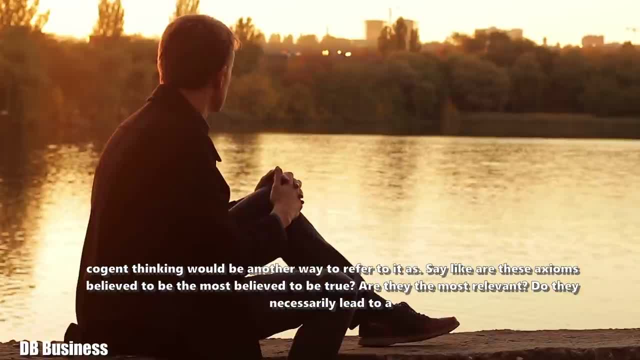 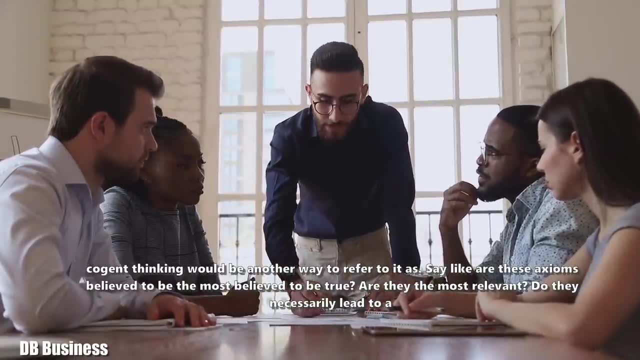 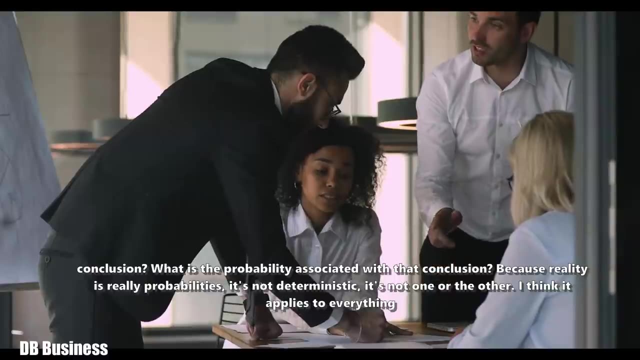 fundamental axioms- sort of cogent thinking would be another way to refer to it- as say like: are these axioms believed to be the most believed to be true? Are they the most relevant? Do they necessarily lead to a conclusion? What is the probability associated with that? 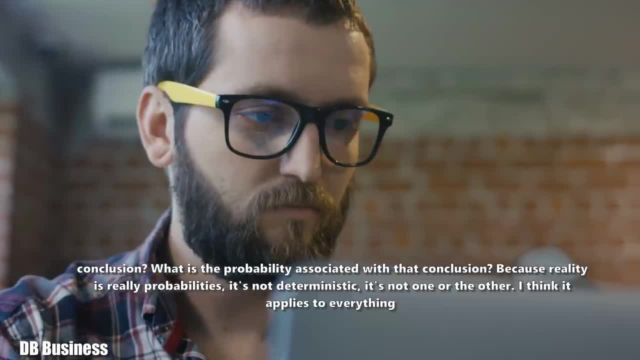 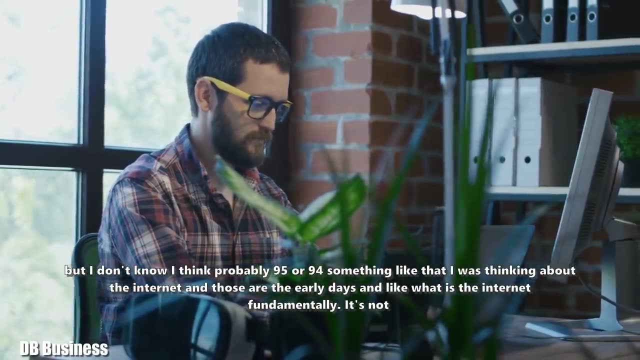 conclusion, The things that, because reality is really probability, It's not, it's not deterministic, It's not one or the other. I think it applies to everything, But I don't know, I think probably 95 or 94, something like that. I don't know. I was thinking. 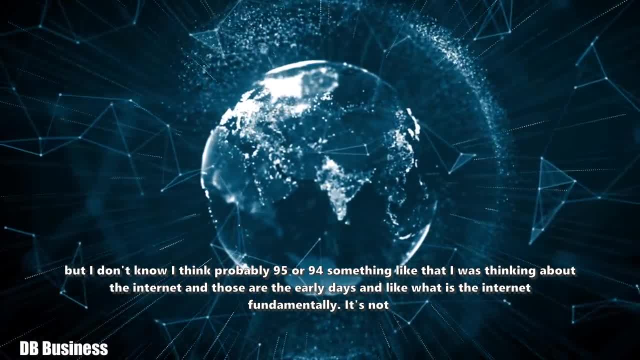 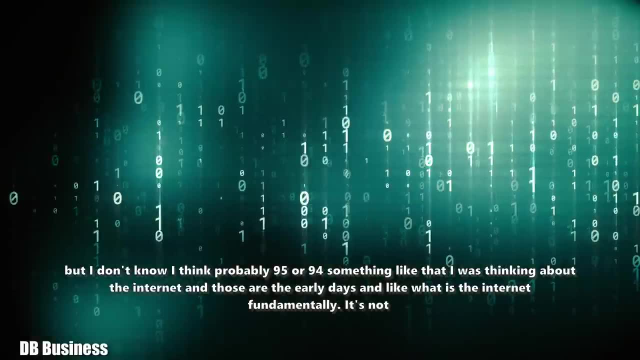 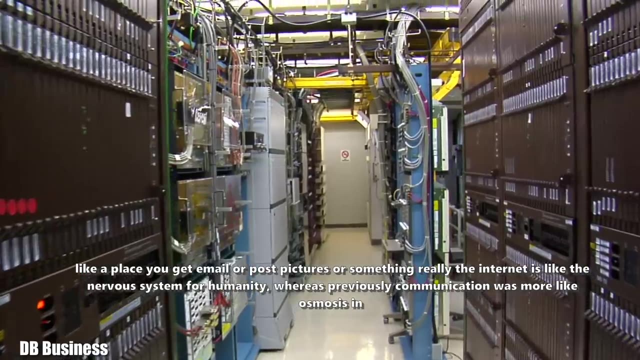 about the internet And those are the early days- And like what is the internet fundamentally? You know it's not. it's not like a place you get email or post pictures or something. Really, The internet is like a nervous system for humanity, Whereas previously communication. 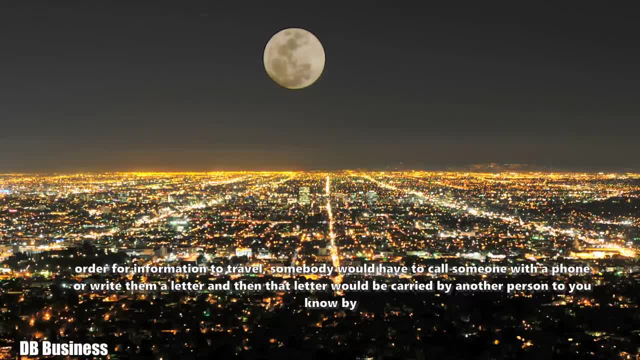 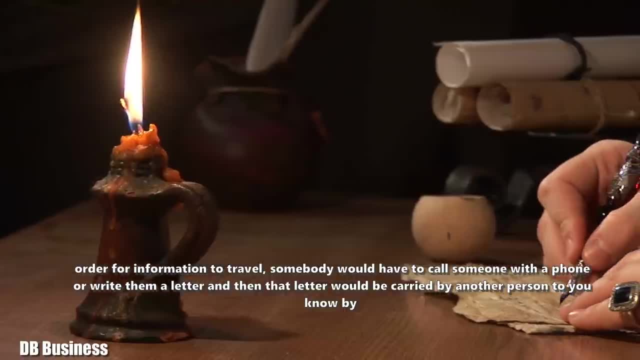 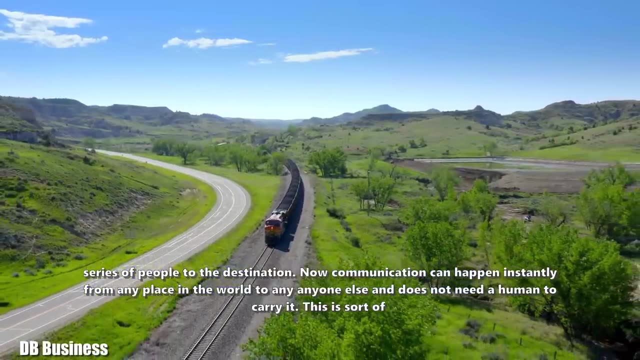 was more like osmosis. In order for information to travel, somebody would have to call someone with a phone or write them a letter, And then that letter would be carried by another person to you know, by a series of people to the destination. Now communication can happen. 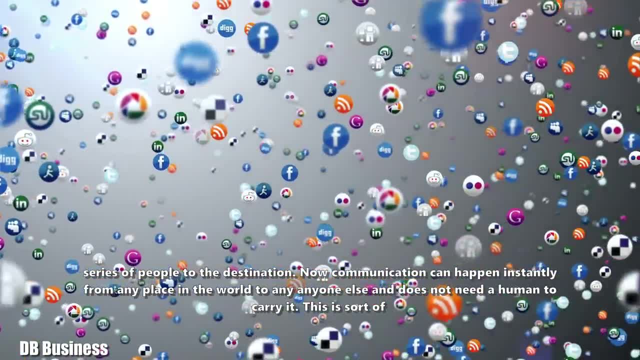 instantly from any place in the world to any anyone else And, just like you said, the internet is like a nervous system for humanity, Whereas previously communication was more like osmosis anyone else and does not need a human to carry it. This is- this is sort of like. 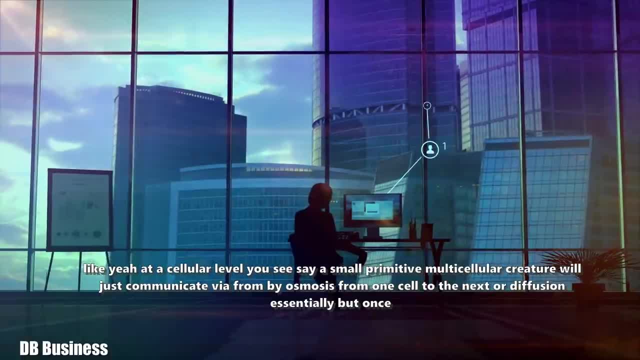 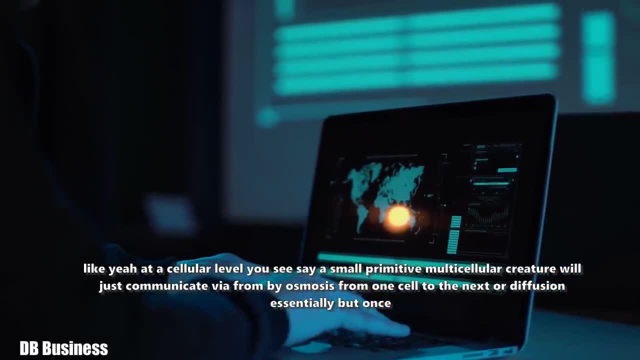 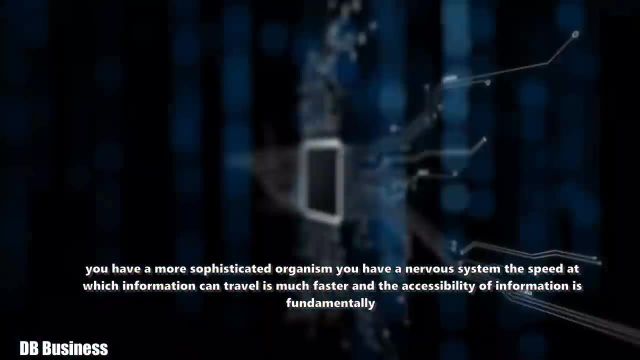 at a cellular level. you see, say, a small, primitive multicellular creature will just communicate via from, by osmosis from one cell to the next, or diffusion, essentially So, but once you have a more sophisticated organism, you have a nervous system. The speed at which information can travel is much faster. 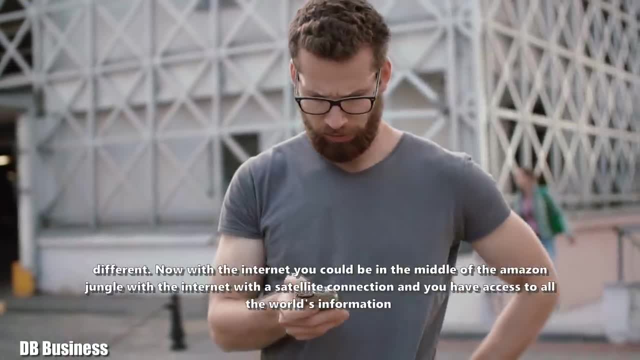 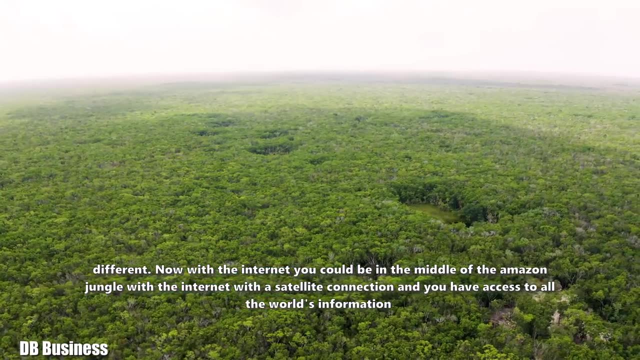 and the accessibility of information is fundamentally different. You know, if you want, now with the internet you could be, you know, in the middle of the Amazon jungle. with the internet, with a satellite connection, and you have access to all the world's information, Whereas previously, even if you lived in the